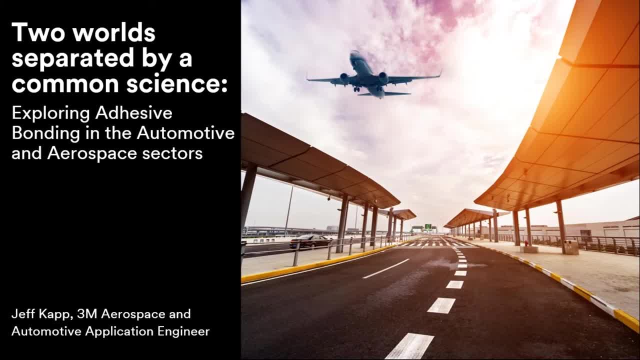 differently to the different markets. So what I'm going to do today is I'm going to walk through the application of adhesives in both aerospace and automotive and compare and contrast the different sectors and approaches. But before I get into the detail of that, I'd like to talk a little bit. 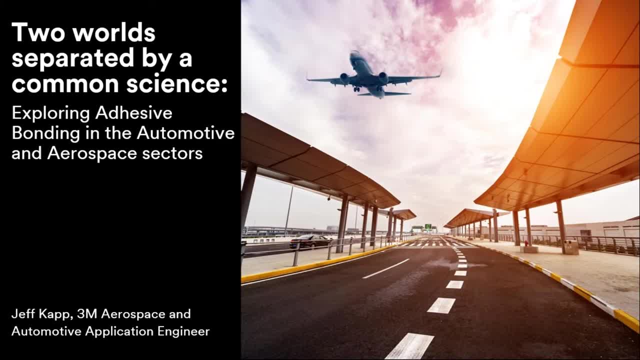 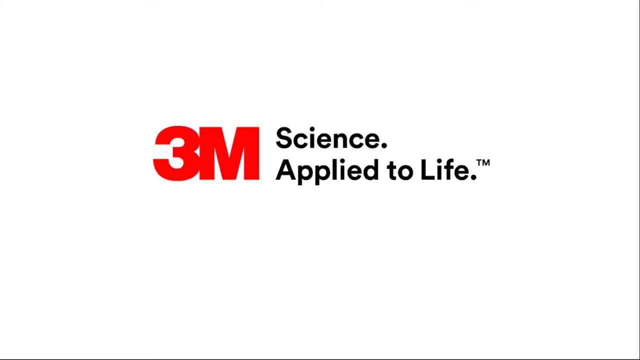 about 3M. If you know nothing else about 3M, it's important to understand that we are a science based company, But we believe that science is just science until you do something with it In all sorts of ways, big and small, we use 3M. 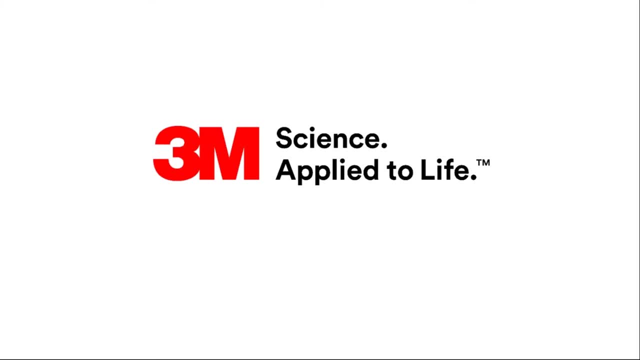 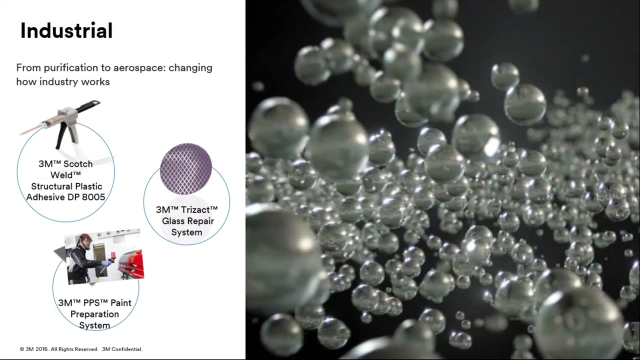 science to improve lives, solve problems by working closely with our customers and also with each other. This is what 3M strives to do every day. 3M is made up of five business groups. Aerospace and automotive is based in industrial and this is our biggest business in terms of. 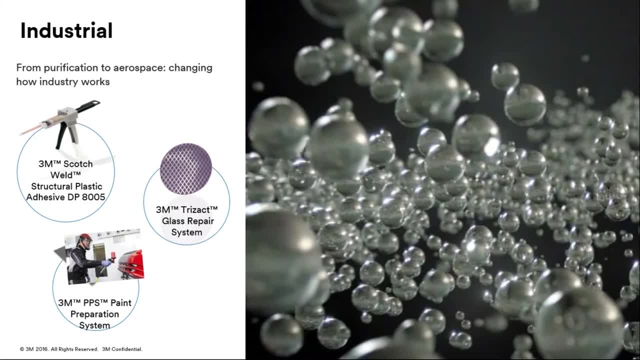 industry. The areas that industrial covers include purifying air and water, from residential to biotherm, pharma and industrial, And also modifying bonding and protecting surfaces in construction and manufacturing. We improve the design and manufacture and maintenance of land. 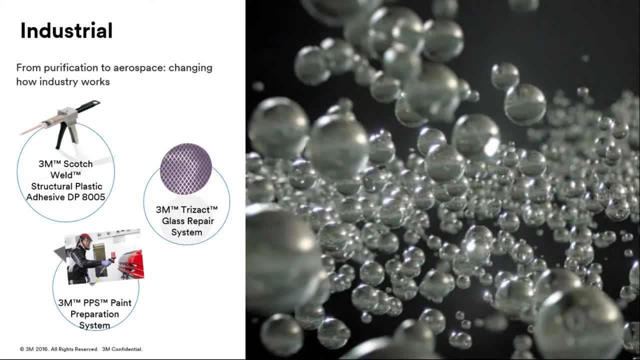 air and water transportation From cargo boxes to babies' nappies. we secure the things that need to stay put. The image that you can see on your screen represents a 3M design. 3M is a 3M glass bubble technology. We are a pioneer in glass bubbles and they're used in a wide 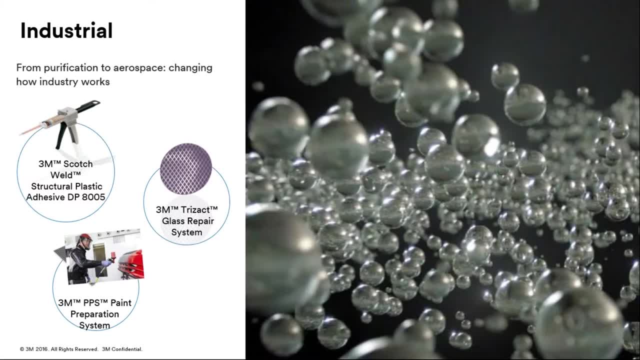 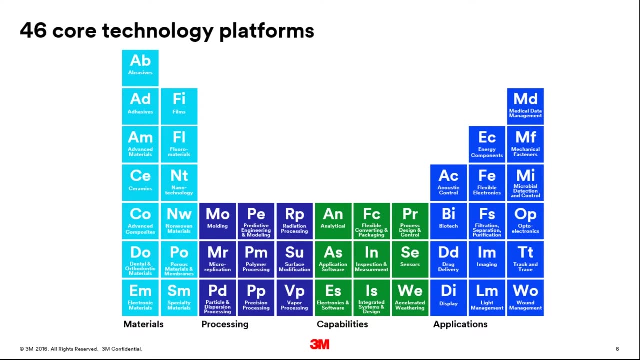 range of industries, from including car and aero parts to reduce weight and lower cost. Unique to 3M is the breadth and diversity of our technology pool, which reflects our uncommon approach to R&D. At 3M we do R&D a bit differently. We separate the R and the D Scientists in our 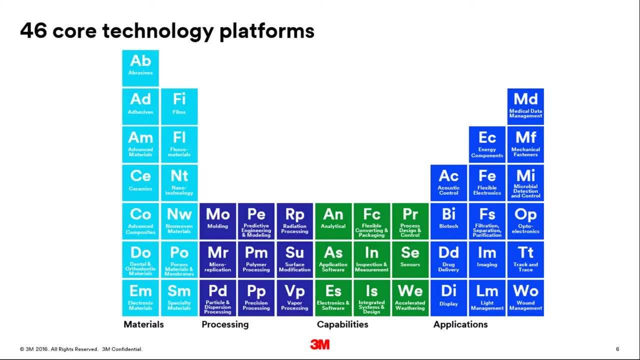 laboratory are free to focus on pure research, looking for unscripted, unexpected opportunities for breakthrough, Whereas those in the development teams that I am within of each of the five business groups then draw upon these core technologies to develop products for targeted markets and geographies. On the screen you can see a representation of our 46 core technology. 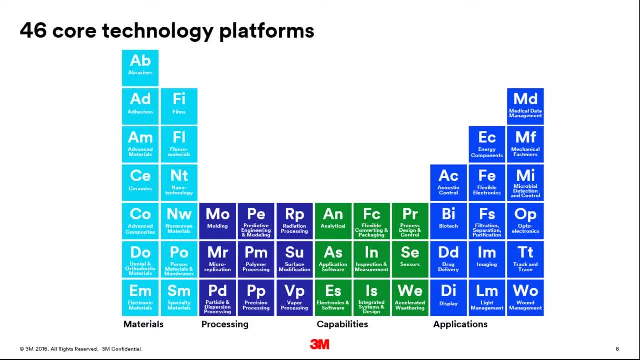 platforms which range from adhesives to abrasives, from sensors to electronic materials. Our team has the uncanny ability to combine and use the technologies in creative ways. That's how a mixing technology originally created for dental crowns has made its way into automotive applications. 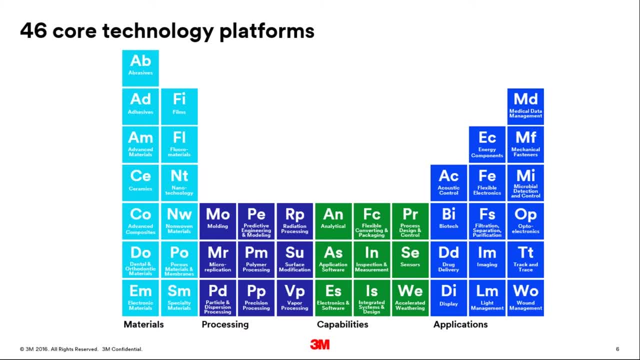 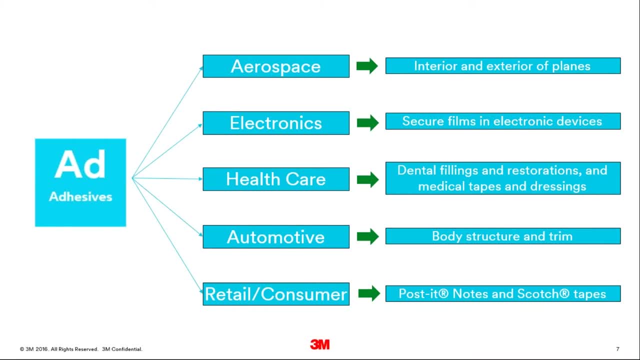 Looking specifically at our adhesive technologies, it's another example of how 3M technology is applied to different markets through our businesses. Because our adhesives are engineered to fit our customers' unique needs, it's hard to find the right adhesives. We're looking to see if this is a good 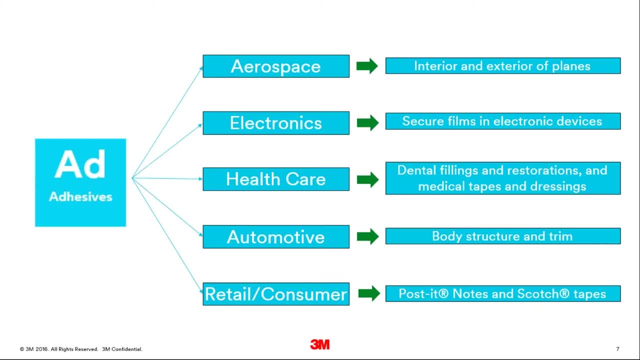 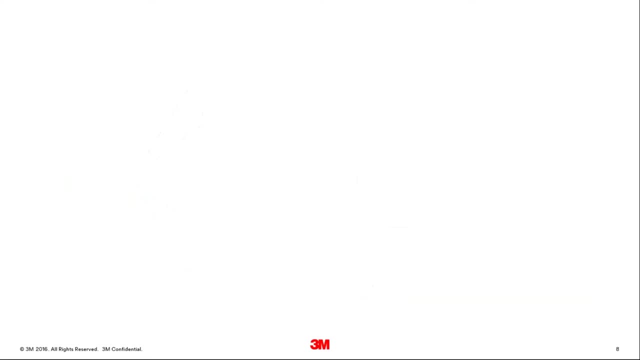 They're using such diverse products as smartphones and dental fillings, through to the aerospace and automotive components that we're going to talk about today. So, before I get started on the presentation, I'd like to understand why we are interested in adhesives. 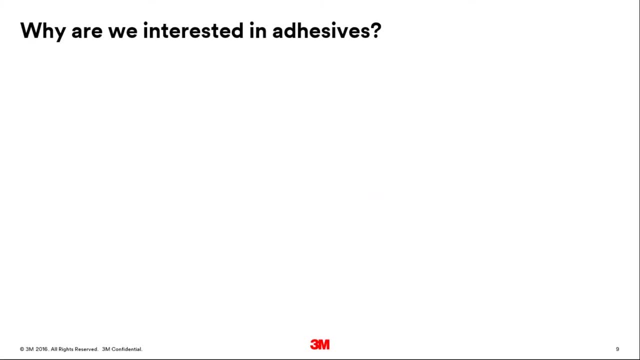 And I use we in a very broad sense here. It may be the adhesives industry, it may be the aerospace industry, or it could just be us here on the webinar. So if you could send in a few suggestions, Okay, we're going to talk about light weighting coming in. aesthetics, come in here. stress. 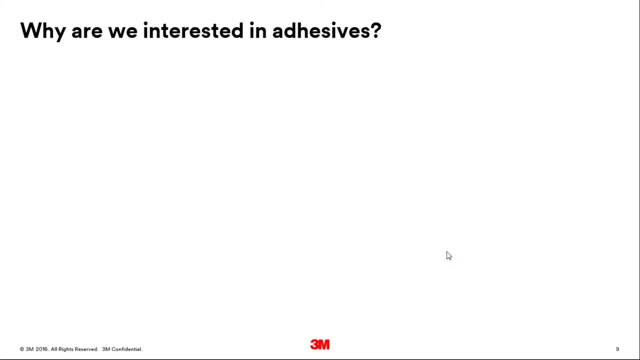 transfer. Okay, I think I can broadly group these in. They come under two headings that I've put here on this slide. First part is about more efficient structures, be that better stress transfer because of the fact we're using continuous joining technique rather than discrete with mechanical fasteners. 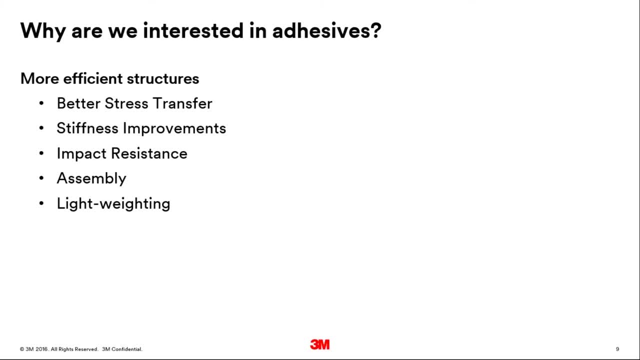 or welds or rivets. Stiffness improvements, Impact resistance is another reason. And assembly- Now that may be the assembly technique, or it might be a neater assembly in order to achieve better aesthetics. But also light weighting is becoming a more and more prominent reason for using adhesives. 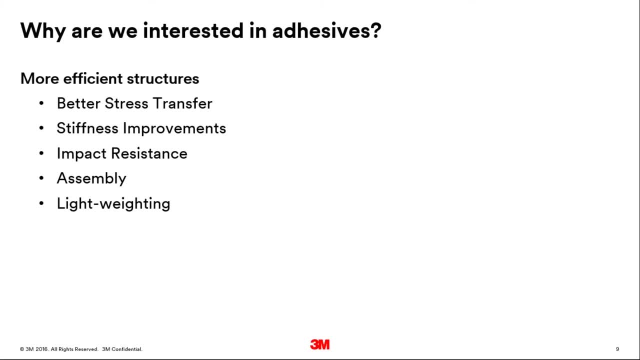 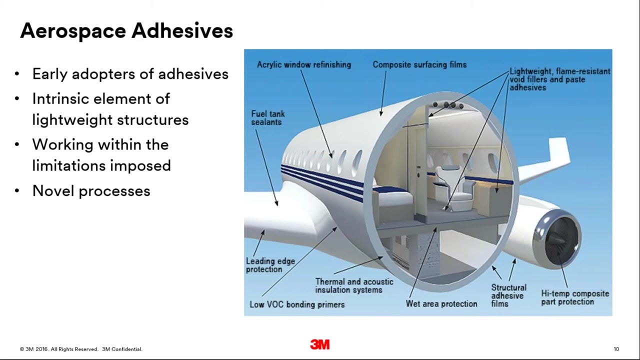 But there is another reason: Because we have to. Quite often welding or mechanical fixings are impossible, Okay, And perhaps may cause stress concentrations on sensitive substrates such as composites. Thanks for your interaction on that. it's very helpful. So, if I start to talk about the aerospace adhesives and the aerospace industry was really 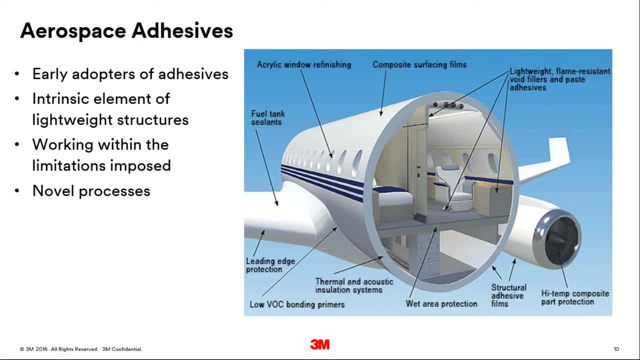 an early adopter, as adhesives are an inherent and intrinsic part of producing a light weight structure. Therefore, the aero industry had to find ways to work within the limitations imposed. Okay, In the early days. I'm talking about limitations in terms of bond gap, tightly controlling. 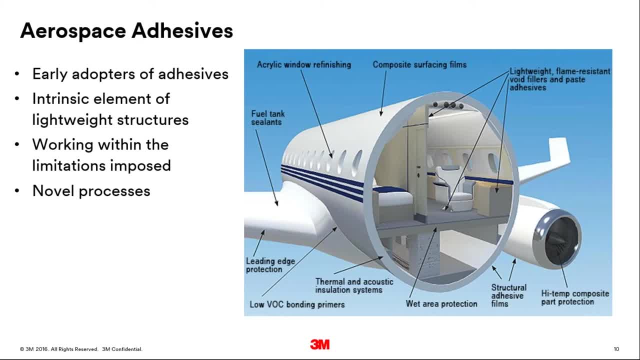 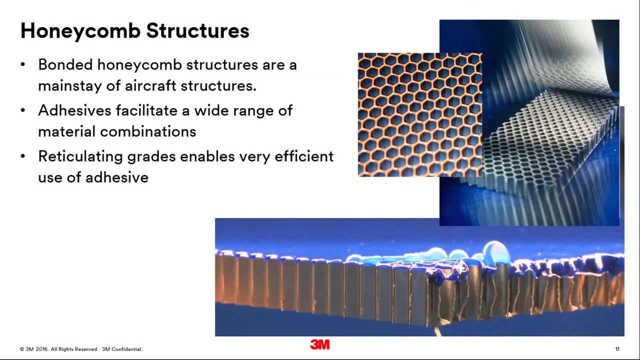 a bond gap, maybe a specific cure cycle or specific surface prep regime, And in meeting these challenges, some very novel processes have been developed along the way. Honeycomb structures are a real mainstay of aircraft structures in that they give us the ability to produce very light but stiff panels. 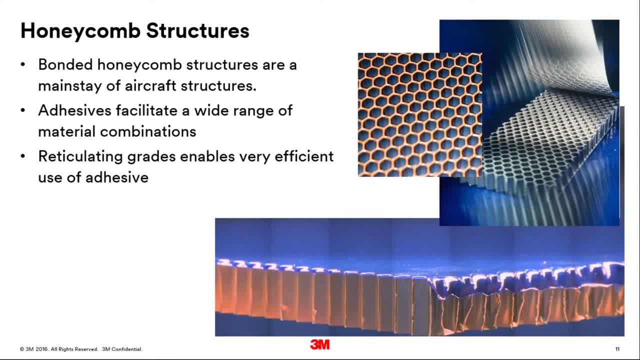 However, we need to join the skin panel to the honeycomb, And adhesives are a key part of being able to do this, But we've got limited surface area and we need to create a variable, very durable bond able to withstand some of the harshest environments. 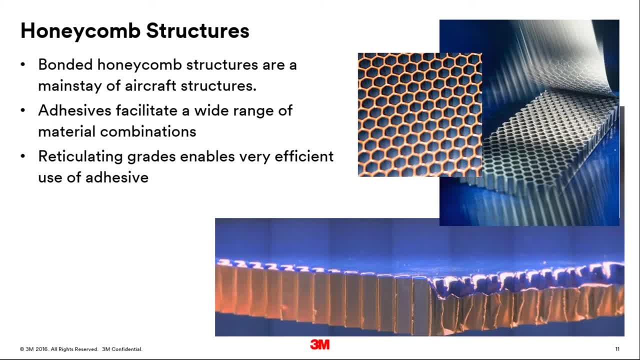 So we developed reticulating grades of adhesives and you can see that simulated down in the bottom right hand corner Where we're blowing air through the molten adhesive or softened adhesive so that it coats the edges of the honeycomb and it creates a filleted joint with no redundancy of the 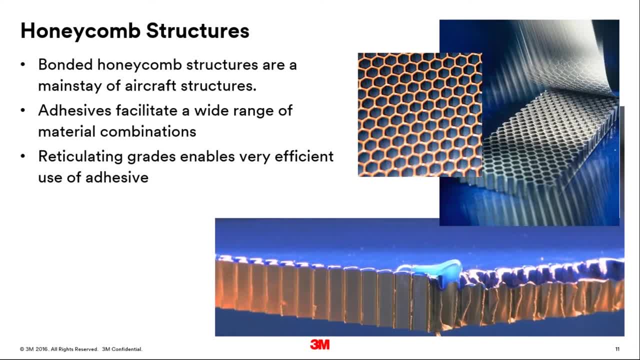 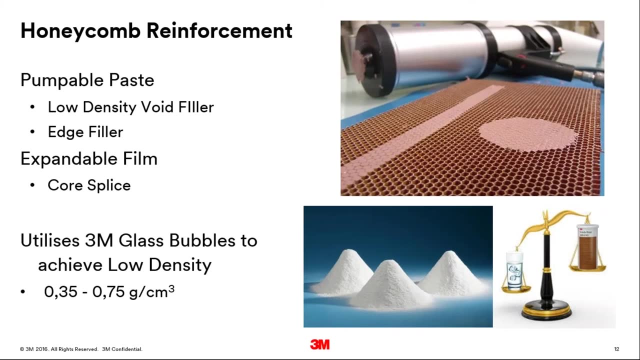 adhesive in the holes in the honeycomb. However, honeycombs have their own restrictions. when we go to join them, We might need to make a T-joint or a corner, or indeed embed a fixing into the honeycomb. Therefore, we've developed grades of low density void filler. 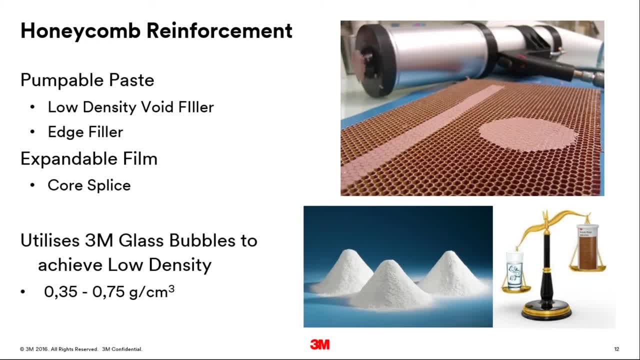 Which can be used to locally reinforce the honeycomb so that we can make a joint. These grades are these low density void fillers are available both as pumpable paste and expandable films, The films being used for areas such as coarse splices or edge finishing. 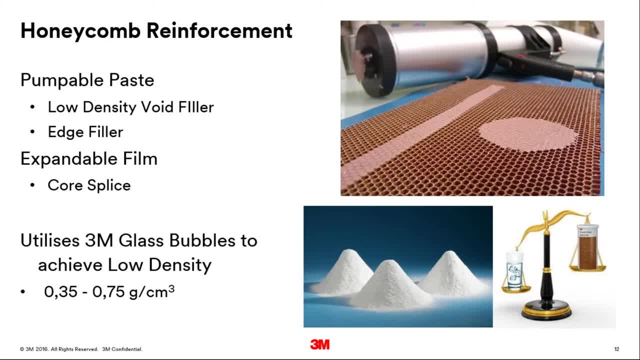 A key component of the low density void filler, In fact, the 3M glass bubbles that I mentioned earlier, enabling us to achieve very low densities but retaining good mechanical properties. In the top right corner you can see one of these structures. I'm talking about a T-joint. 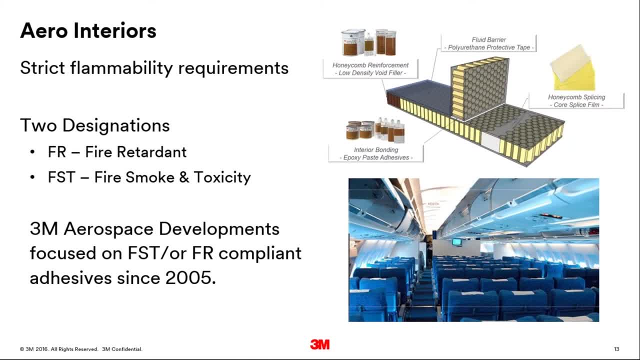 with a coarse splice, And this is an example of an aero interior structure, But however, it's a very simple example. You can imagine that an overhead locker or a gantry will require some quite complex structures And this in turn drives some quite innovative approaches and demands on the joining solutions. 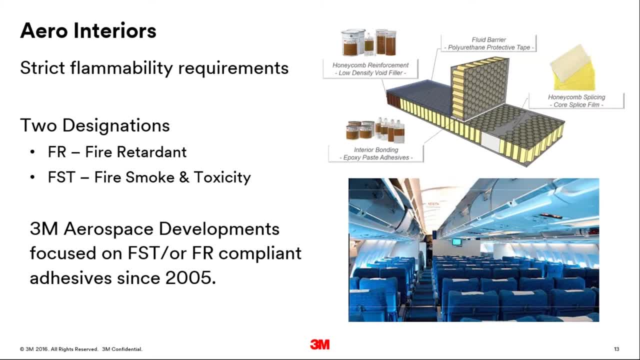 However, the interior market also gives a further challenge in that it has very strict flammability requirements, And this has been a particularly important development area over the last few years, Unfortunately related to disasters such as that at Manchester airports. There are different regulatory requirements in different regions. 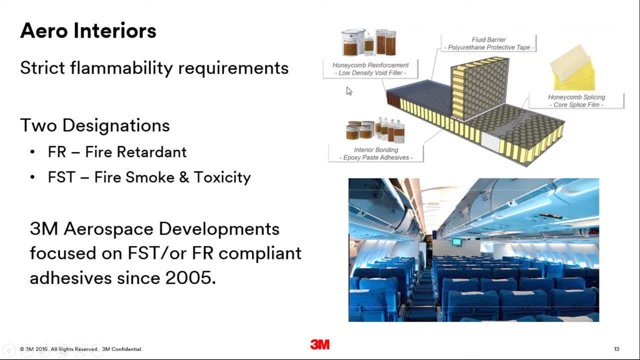 And an aircraft manufactured in one location are actually controlled by the regulations of the country that they fly into, So therefore it tends to be the most stringent regulations that are applied. There are two designations: fire retardancy, which is to do with managing the burn of a. 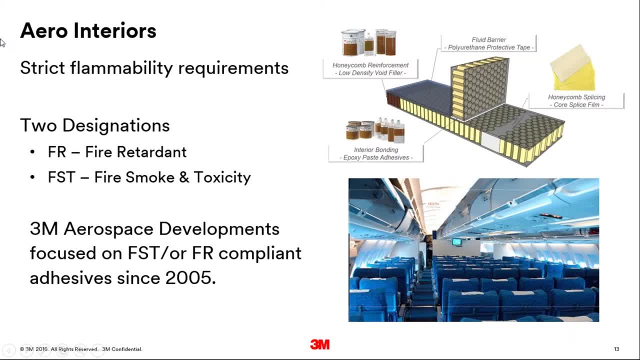 product And the spread of fire and fire smoke and toxicity. FST, which deals with the chemicals produced when something burns, when a product burns, And 3M. Aerospace Developments have focused on FST or FR compliant adhesives for interiors. 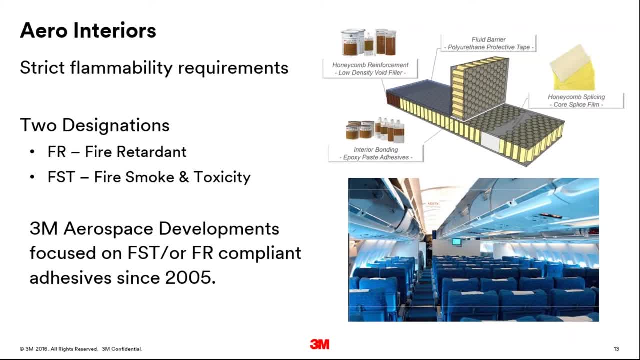 since 2005.. And in 2007,, we launched an innovative product which is a flexible epoxy technology 7246-2, as the first FST FST compliant non-halogenated paste adhesive for the interiors market. 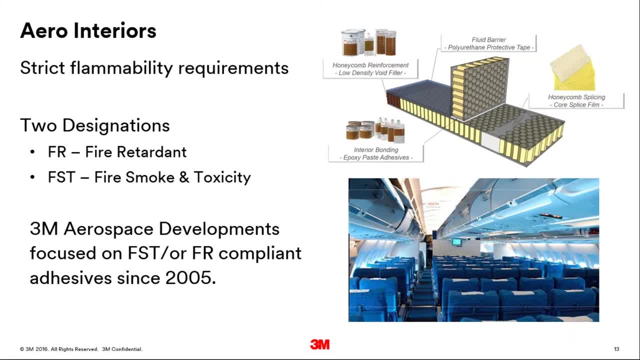 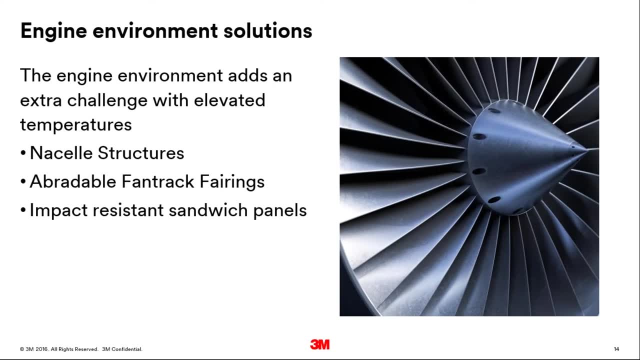 Another application that delivers an extra challenge is the engine environment, where the adhesive bonded joints need to perform at elevated temperatures, And our adhesive technologies are used in a wide variety of structures, such as the NAR cells with air inlets, bypass ducts and thrusters. 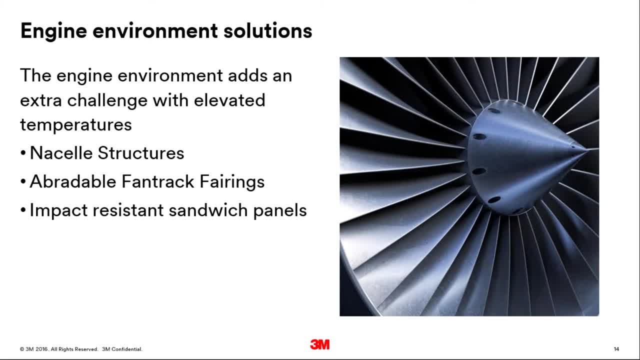 And also sound suppression sandwich panels. Low density void fillers are used as fan track liners within the engine casing, where we apply the low density void filler and then allow the tips of the blades to wear away some of the fan track liner to create a very high tolerance gap and enabling very high 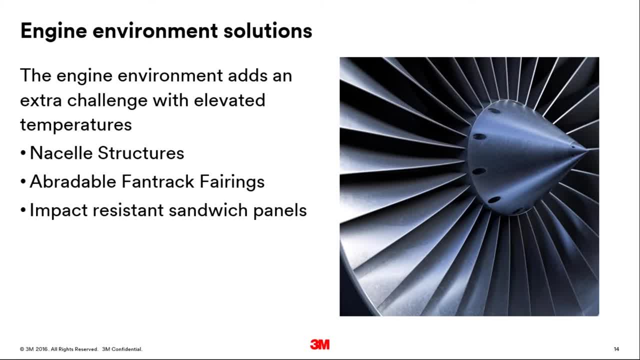 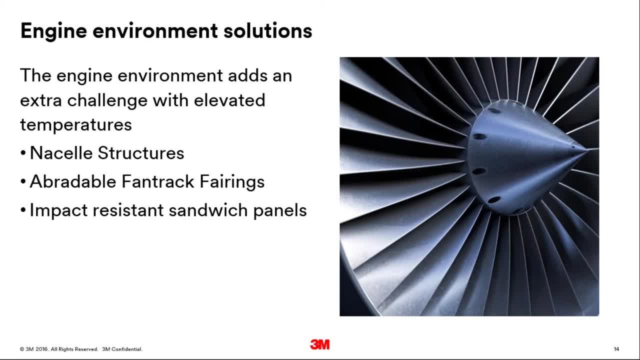 and low density void filler technologies. These enable us to deliver solutions for managing blade release events. But the aerospace market isn't standing still. It's evolving into more and more demanding applications, be that loading temperature, durability or, in fact, weight reduction. 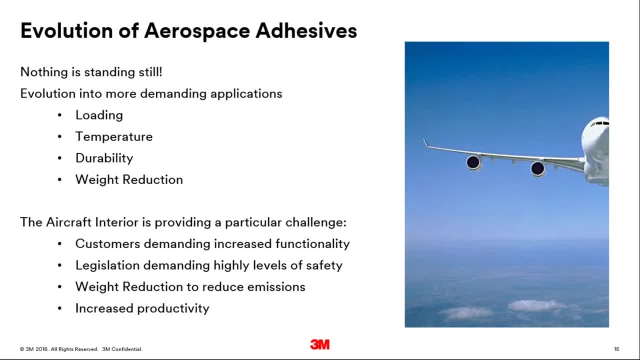 And the ever-growing need to make aircraft lighter And the aircraft interior is providing a particular challenge, with customers- be that the end user or the aircraft manufacturer or the airline- demanding increased functionality, legislation demanding higher levels of safety and weight reduction to reduce emissions. 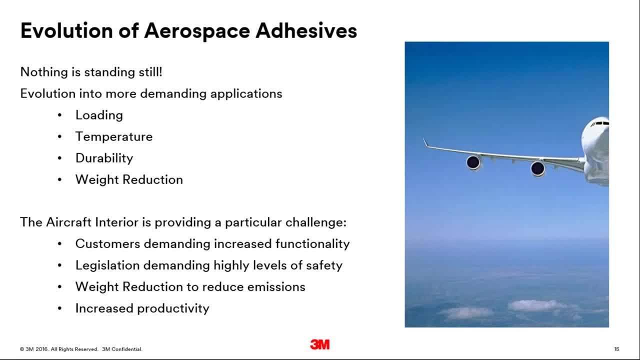 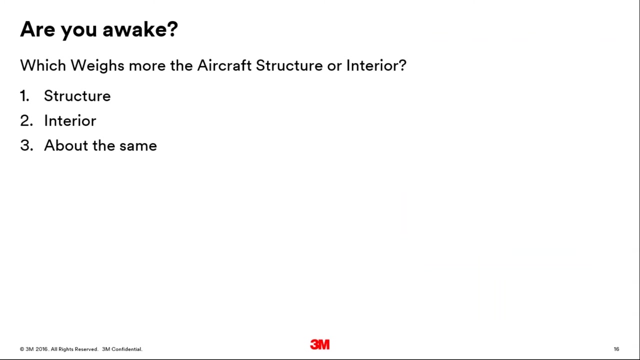 Coupled with that, aircraft are at the highest build levels yet, which is demanding increasing productivity and some new methods of production. I'm going to test who's awake now, in that I'm going to open up for a poll. So which do you think weighs more, the aircraft structure or the aircraft interior? 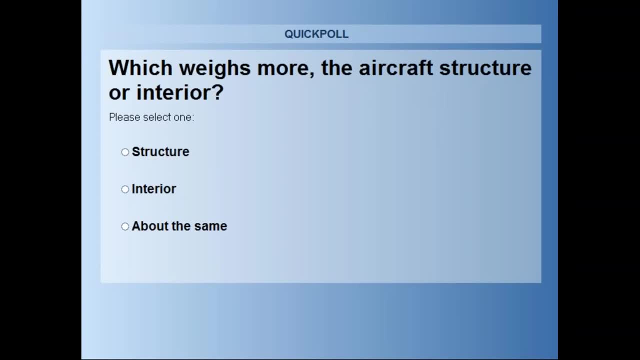 Or third option. are they round about the same? I've got some votes coming in. Oh, we've got some smart people on the line. Yeah, we've got 80% choosing the interior. Absolutely, I'd agree with you. 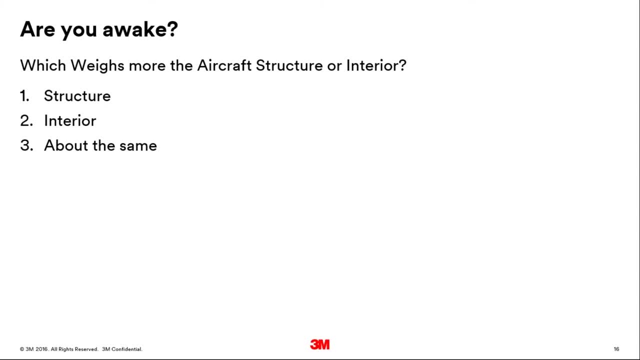 But interestingly enough, that's not dissimilar from the automotive environment, where we're all demanding much, much more from the interior. And then the other one is, of course, the top of the car, which is an incredibly high -end model. 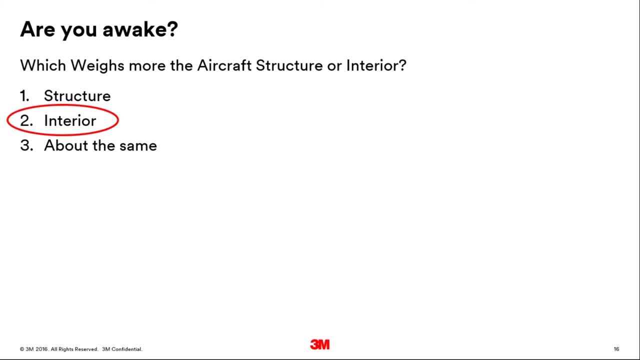 And that's the front end. That's the rear end, which is the front end. So we've got a lot of different aspects to choose from, But the top of the car is the top of the car And the rear end is the top of the car. 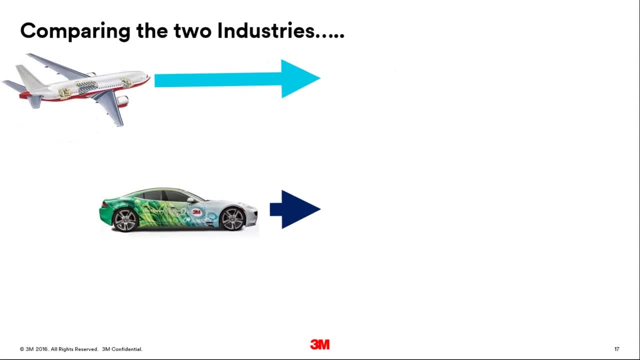 So we're not going to be talking about the entire car, but the entire car. So we're going to be talking about the entire car. The two different things will be a bit more clear about how much the difference is between the features, the features of the car, the features of the car and the features of our. 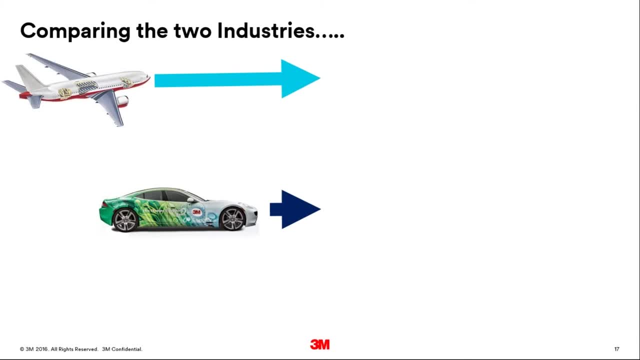 vehicle and with the safety requirements as well, driving the weight up. So if I start to compare the two industries now, As demonstrated, the aero industry has really embraced the use of adhesives, wings- sorry, pardon the pun- watching, learning and adopting some new techniques and developing. 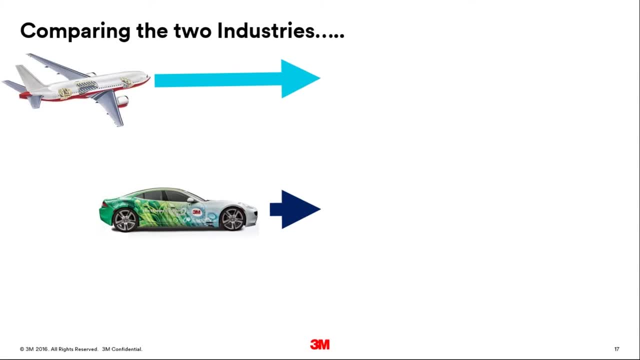 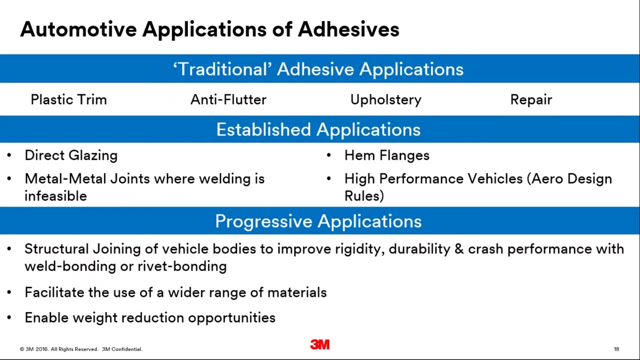 new approaches. This slide here gives an overview of the use of adhesives today in the automotive industry. We've got those traditional applications that have been around for a hundred years or so: plastic trim or wood trim as it was back in the day- anti-flutter to stop two metal panels. 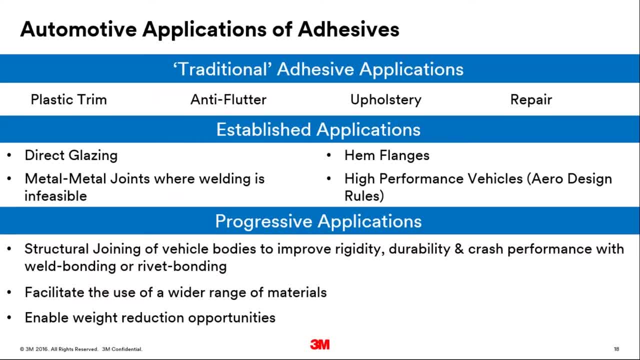 knocking together and producing an unpleasant noise. upholstery and also repair when we damage our vehicles And we've got the established applications over the last decade or so where we've moved into direct glazing of vehicles, so we're bonding the windscreen directly into the 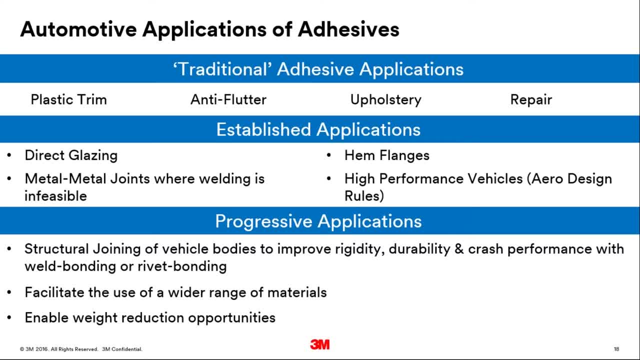 vehicle body. We also have hem flanges where we're joining the inner and outer panels of a door in order to produce a stiffer, lighter structure with better corrosion resistance. Adhesives are also used in metal to metal joints where welding is infeasible. 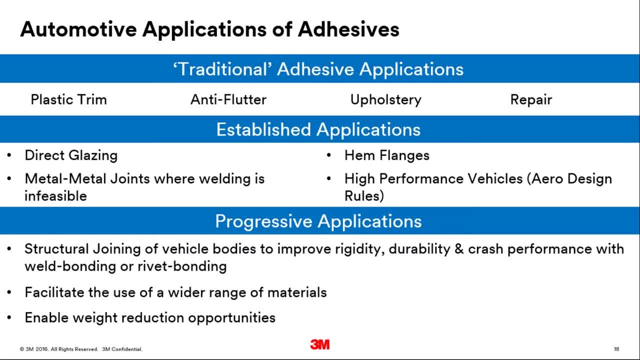 where you can't get the spot weld done in and in high performance vehicles, really following the aero design rules and adopting the aero products. But we're now moving in to what I would call progressive applications, where adhesives are being used. 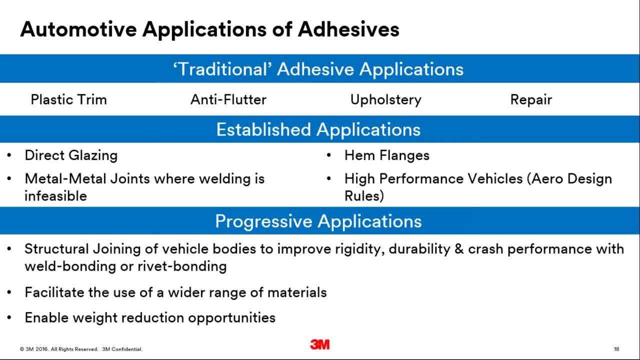 for true structural joining of vehicle bodies to improve rigidity, durability and crash performance, And this is due to the fact that we've got a lot of adhesives that have been used for a long period of time. We're also seeing adhesives used to facilitate a wider range of materials and 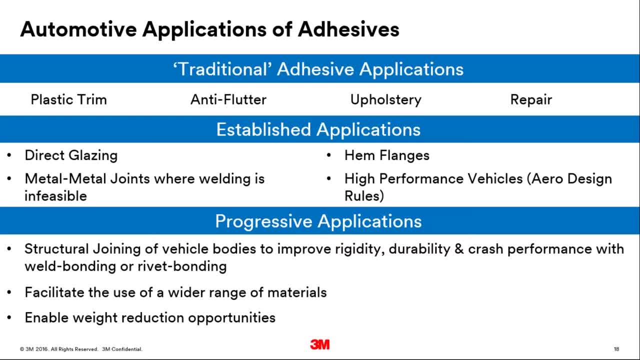 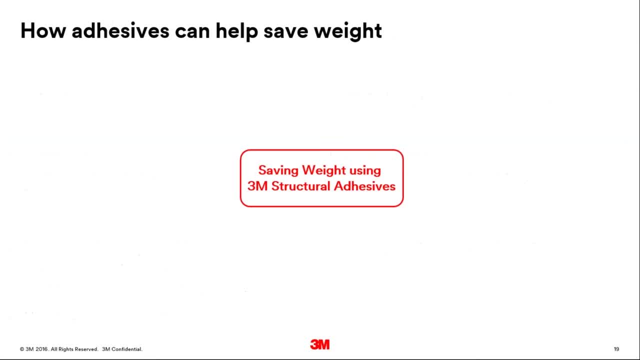 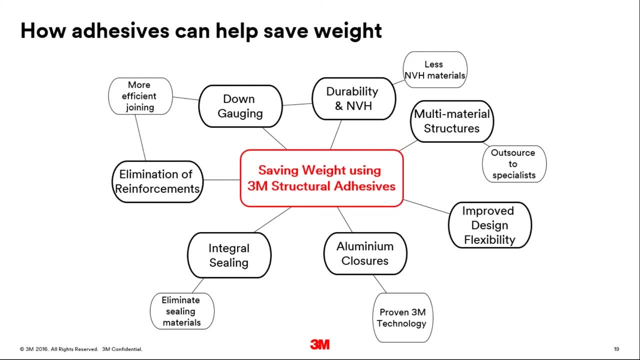 enable weight reduction opportunities. The diagram appearing on your screen now is from a presentation that I give, specifically looking at how adhesives can be used to save weight And, as you can see, it opens up a multitude of options. We might use adhesives to enable us to down gauge a panel. We no longer need to have that extra. 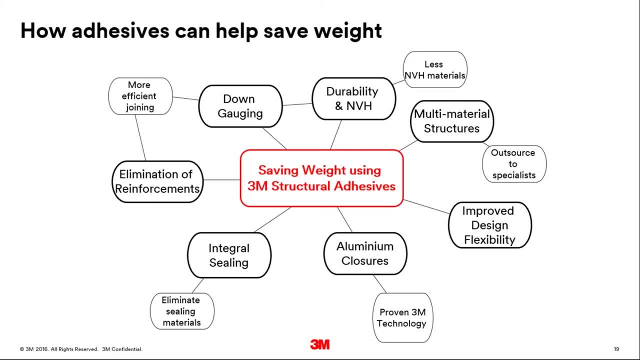 material there to facilitate a mechanical fixing or a weld, so we can down gauge through the more efficient joining technology. This may also enable us to eliminate some reinforcements in joint areas, again by better load transfer. Adhesives also offer us the opportunity to integrate the ceilings, So no longer do we have to join and then seal over the top, but the adhesives. 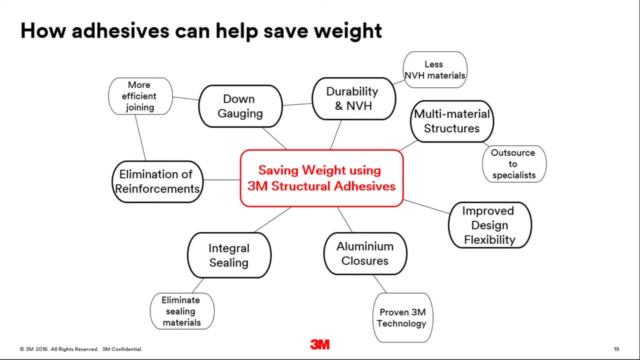 does the sealing function as well. But what I'd like to focus on today is multi-material structures: How adhesives can be used to enable us to make a hybrid structure. The vehicle body is a complex structure, and, while a great deal of expertise has been established in spot welding of steel, 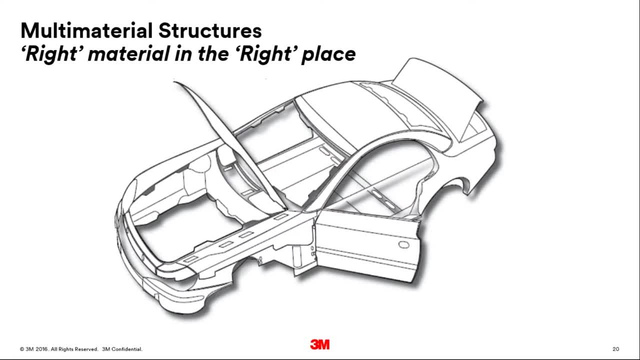 as performance demands are increasing, designers are looking towards alternative materials for greater scoping design freedom. The latest grade of high strength steels can enable slimmer sections and higher loading, while aluminium skin panels can lighten hang on parts and enable hinges to be more compact and knock on weight savings. Composite materials can be used where there's. 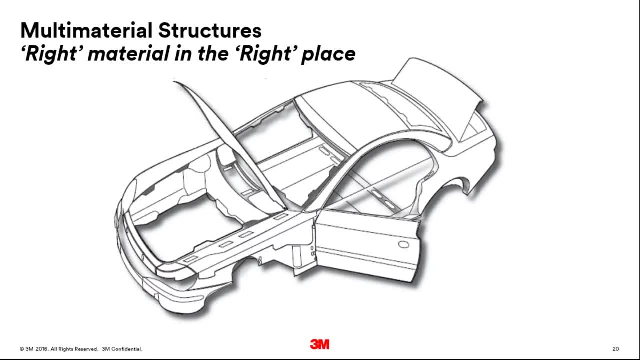 a high degree of part integration. part integration, such as the spare wheel, well, or tailgate, for example. Using the right material in the right place opens the door to ultra-efficient vehicle structures, But it can clearly be seen that these type of structures are a challenge in terms of 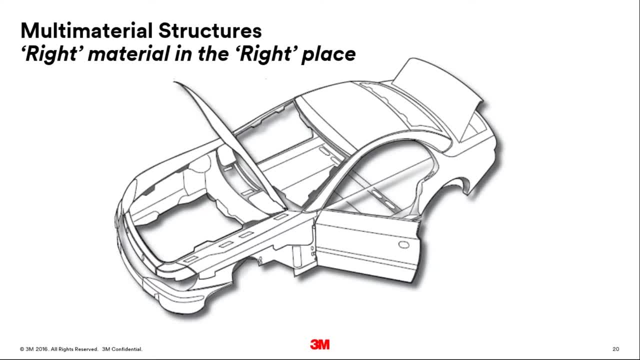 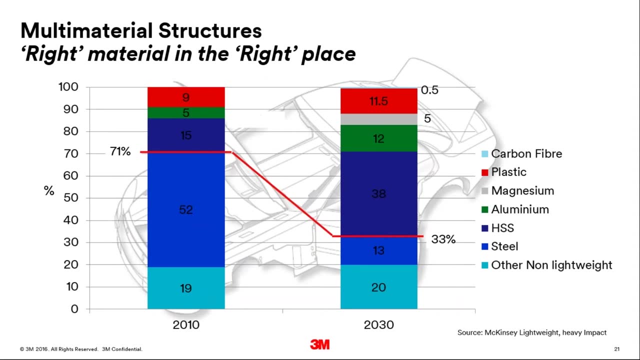 joining, representing a very broad spectrum of mechanical, thermal and corrosion properties. The chart here from McKinsey projects material usage trends forward into 2030. And shows a very unfamiliar composition compared with today, with no materials in inverted commas accounting for up to 67% of the body structure. So this implies that by 2030, a maximum 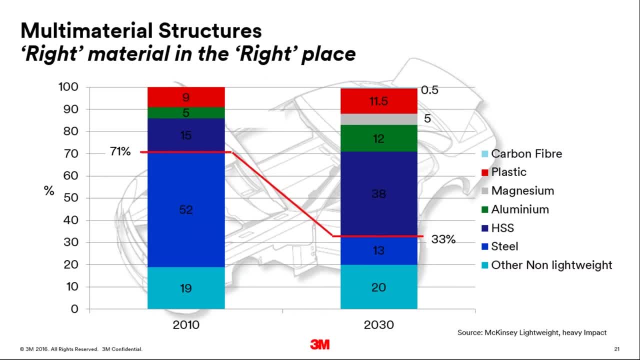 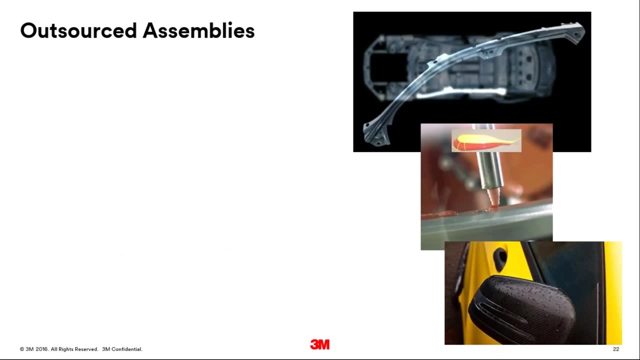 of a third of the body structure will be easily joined by the conventional spot welding which is so well established today. Use of these alternative materials also gives a further challenge, in that much of the expertise resides in the supplier. base. Adhesives again can be used. 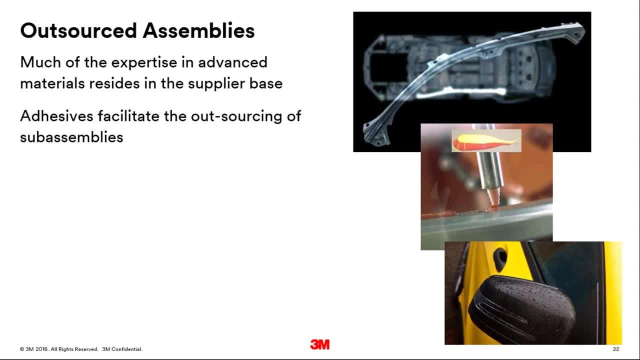 to facilitate this in the outsourcing of sub-assemblies, providing a low skill and investment approach to joining and enabling the sub-assembly to be assembled at the outsourcer and then introduced to the vehicle either at body in white or final assembly, And 3M have invested in 2K adhesive technology and structural adhesive films which allow these. 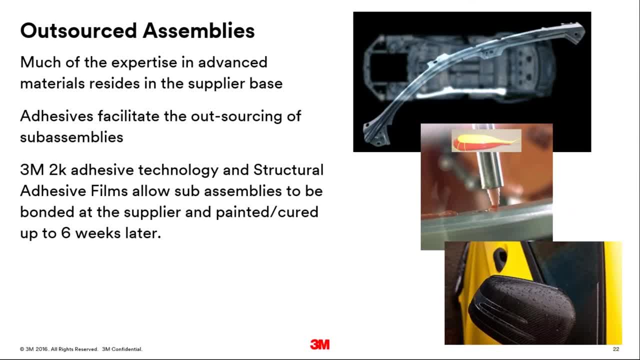 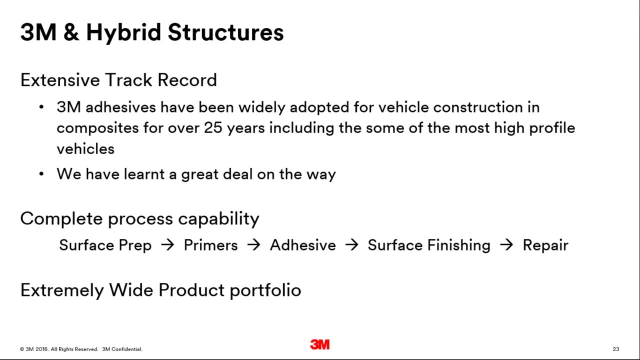 sub-assemblies to be bonded at the supplier and painted or cured up to six weeks later at the OEM in their paint bait cycle. In terms of 3M and hybrid structures, we have a very extensive track record. 3M adhesives have been widely adopted and they have been used for a number of reasons. 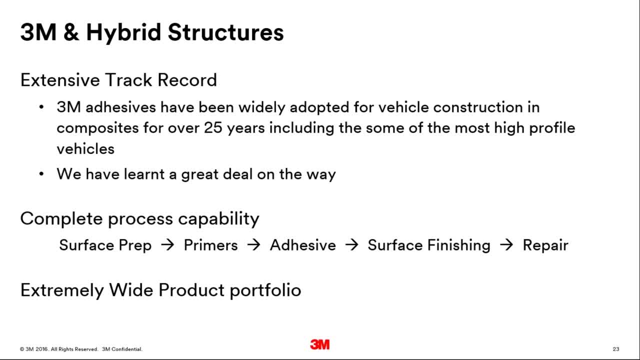 3M adhesives have been widely adopted and they have been used for a number of reasons. We've opted for vehicle construction with composites or hybrid structures for over 25 years, including some of the most high profile vehicles. We've learned a great deal along the way. 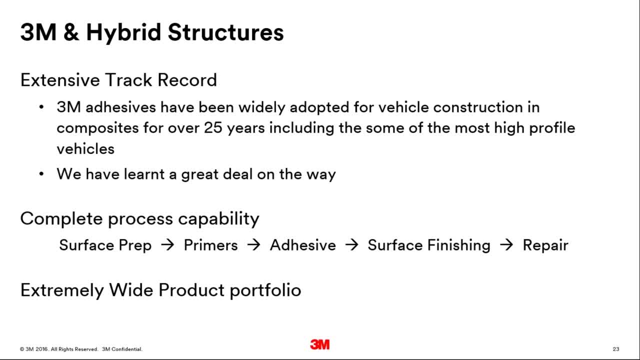 As I highlighted earlier on, 3M has an incredibly broad product pool and technology pool, enabling us to offer complete process capability, from surface prep and primers, through the adhesive, to surface finishing and then repair of the vehicle. We've also offered an extremely wide product portfolio in terms of adhesives. 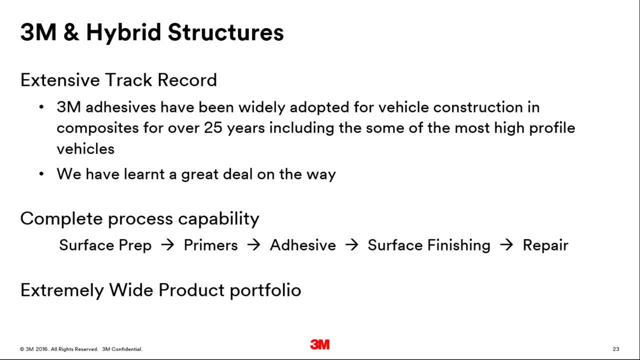 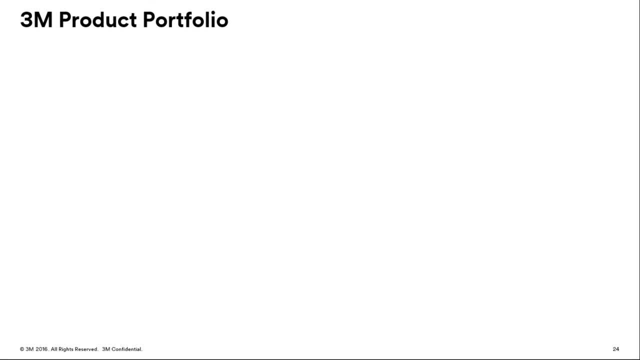 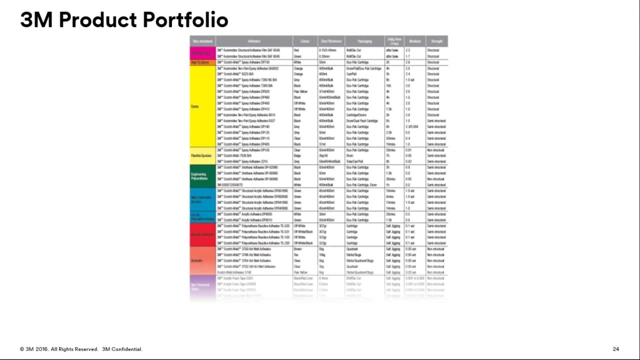 And for your convenience, today I've narrowed this down to just the basic 50.. No, don't worry, I'm not expecting you to read that slide, But it does give an idea of the breadth of product that is necessary in terms in when you're producing a hybrid structure. 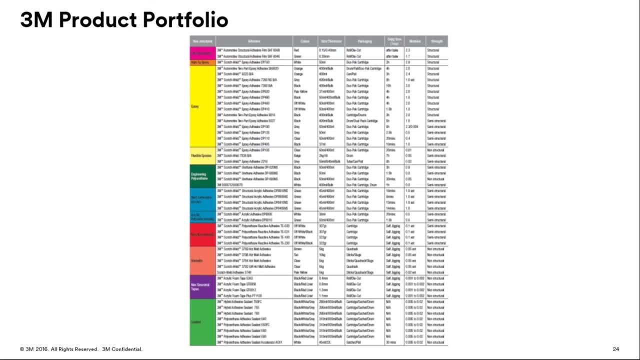 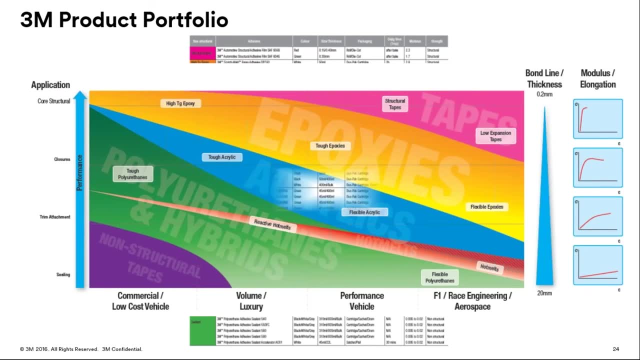 So what we've done is we've tried to boil this down into a domain plot. On the far left you can see the performance of the product moving from ceiling through trim attachment to closures and then into the core structure. And on the x-axis we had the application right the way through from commercial low cost vehicles to 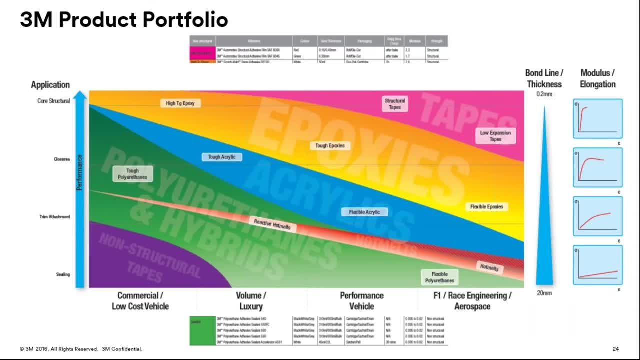 Formula One and race engineering and the aerospace applications. And on the far right there I've given some examples. 3M adhesives have been widely adopted and they have been used for a number of reasons: Impressions of stress-strain curves, Again highlighting the difference in mechanical 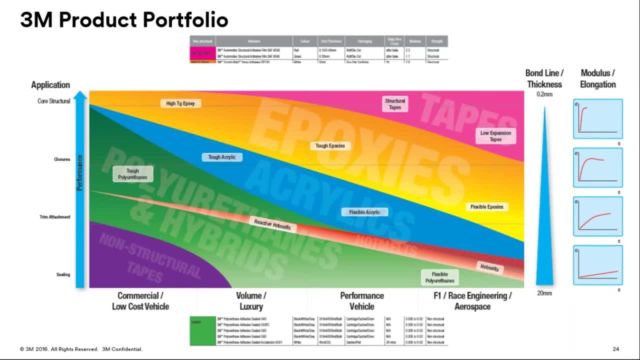 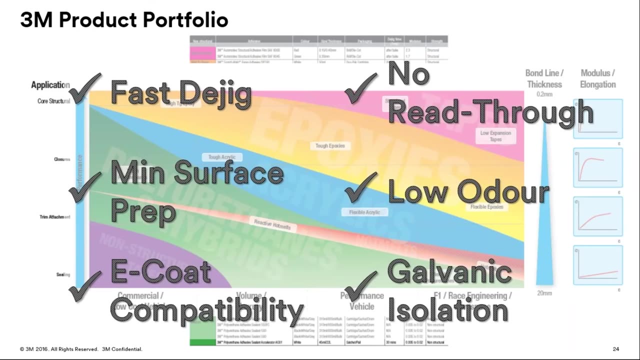 properties that are demanded through hybrid vehicle construction. But it's not all about mechanical properties. There are processing requirements, such as fast de-jig. We also demand no read-through, So this is eliminating any kind of bond line read-through onto the A-surface of the vehicle. Minimal surface preparation, low odour compatibility. 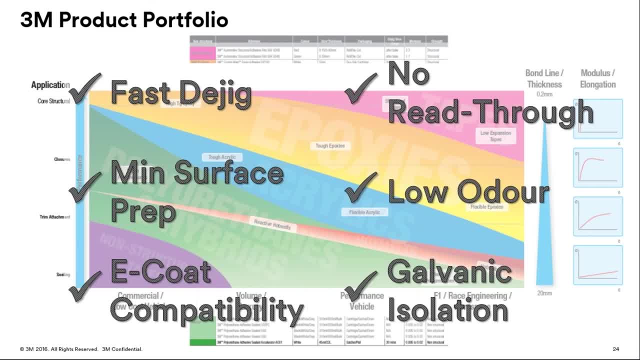 with ECO. So currently every vehicle will go through 180 degrees for half an hour for the ECO bake And also galvanic isolation, and that we need to ensure that these multitude of different materials are not setting up corrosion cells. Now hybrid construction has really moved along in. 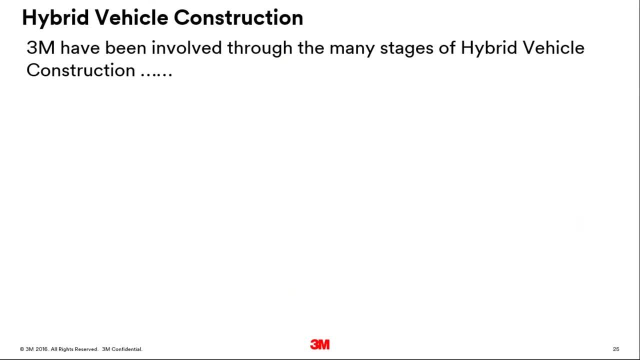 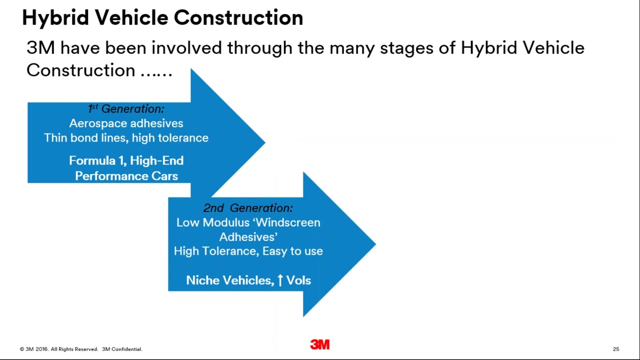 the last 25 years that we've been involved with it. I've called the first generation the adoption of aerospace adhesives. We then saw an evolution into much more, much easier to use products, with some vehicle manufacturers adopting low modulus windscreen type adhesives with a high bond gap tolerance- very, very easy to. 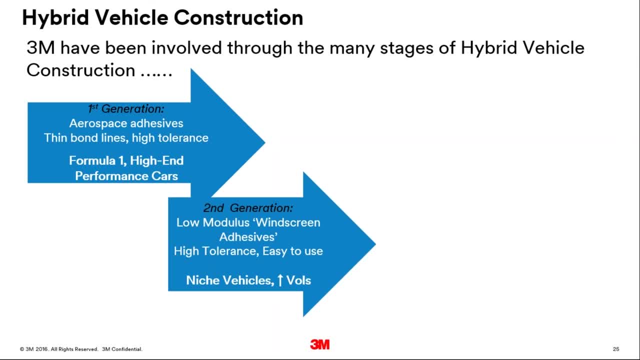 use and surface tolerant. This enabled hybrid construction to be used in slightly higher volumes, But it does not get the best out of your high performance material in terms of stiffness and load transfer. Therefore, in recent years, we've moved over to a combined approach using high toughness core. 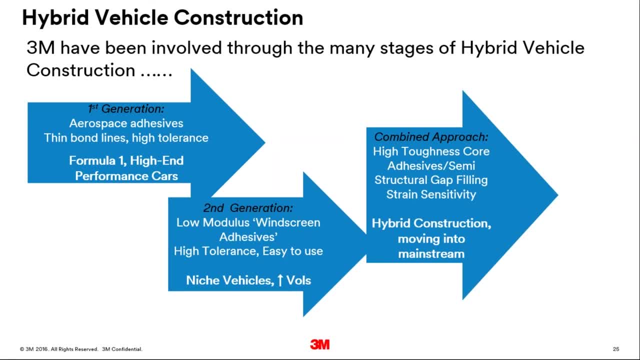 adhesives and then semi-structural gap filling adhesives in less demanding applications, all the time respecting the strain sensitivity of the high performance substrates such as composites. And this is moving hybrid construction into the mainstream, And we've seen a number of manufacturers recently incorporating some quite exotic materials into what you would call mainstream vehicles. 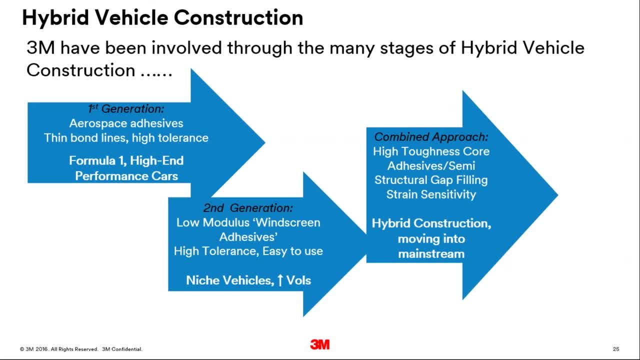 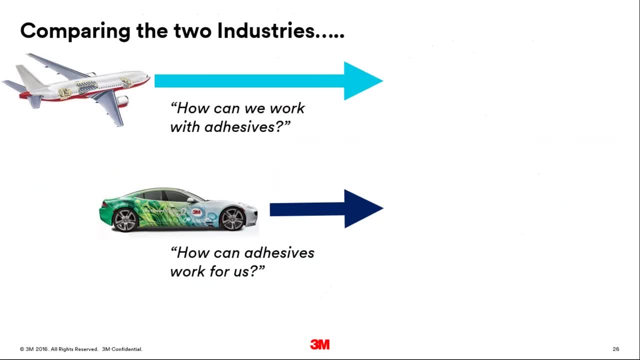 So now I feel that we've moved through the two industries well enough to start kind of grouping the way they work with adhesives. With aerospace we've really seen the specification or performance driven approach, Adopting the adhesive that gives the level of performance needed for the adhesives. 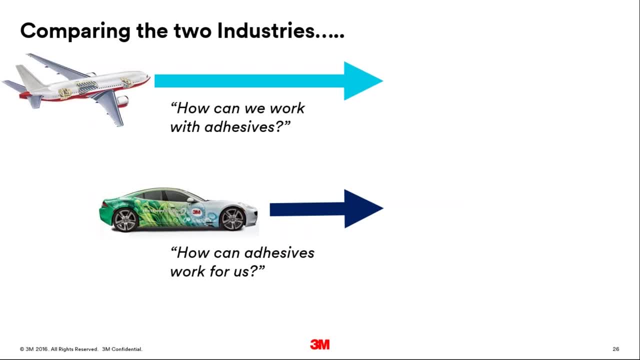 And then we've moved through the two industries well enough to start kind of grouping the way they work with adhesives. With aerospace we've really seen the specification or performance driven approach, Adopting the adhesive that gives the level of performance needed for the adhesives. 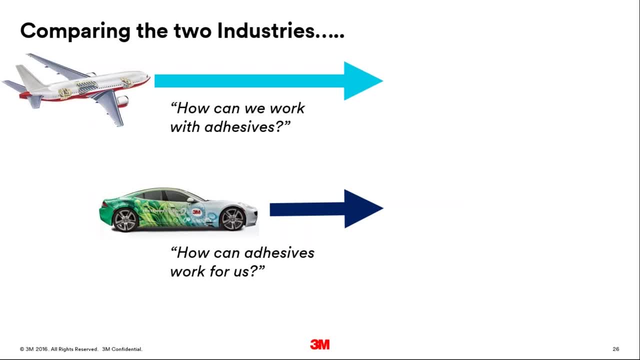 And then designing a process around that to suit the needs of the product. So it's really kind of saying, OK, we're going to use adhesives, Now how can we work with these adhesives? Automotive has taken a slightly different approach in what it's demanded from the adhesives industry, saying, OK, we can see the need for adhesives. 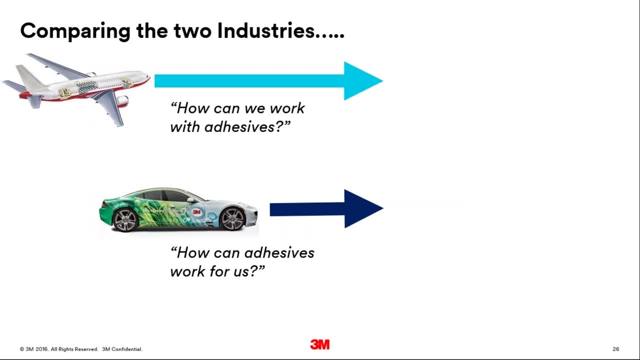 but how can we make these adhesives work for us in terms of not changing the structure too much or not changing the infrastructure too much in terms of the manufacture of vehicles? So I'm going to compare and contrast the adhesives. selection criteria. 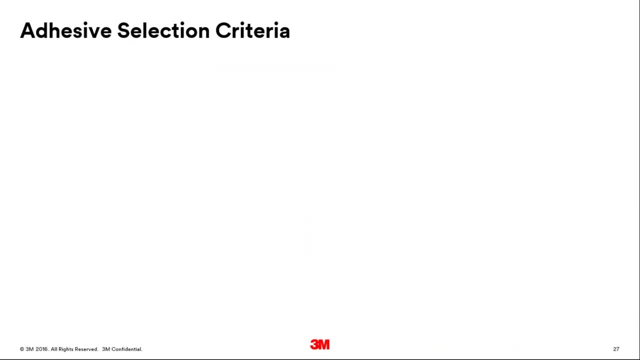 Little bit of tongue in cheek, so bear with me on this one. Please don't get offended. In terms of requirements, let's start with surface preparation. Aerospace will quite happily take on abrasion primers and all sorts of exotic surface preparation where the automotive customer will come to us and say: well, the panel's got oil on it. 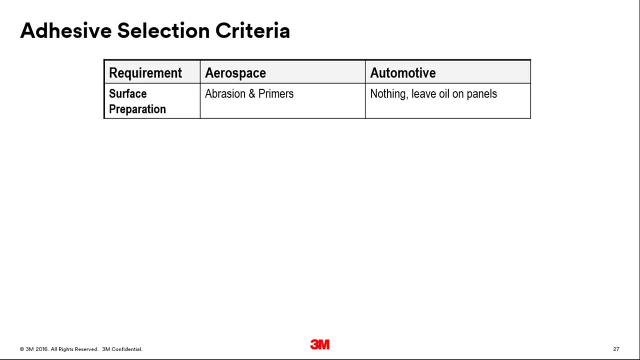 We don't want to take it off Now. give us an adhesive that will bond to it. In terms of bond gap, we need to carefully control to a tight tolerance the bond line that we're providing for our aerospace customers. Automotive customers, in contrast, will want good bead stability and gap fill. 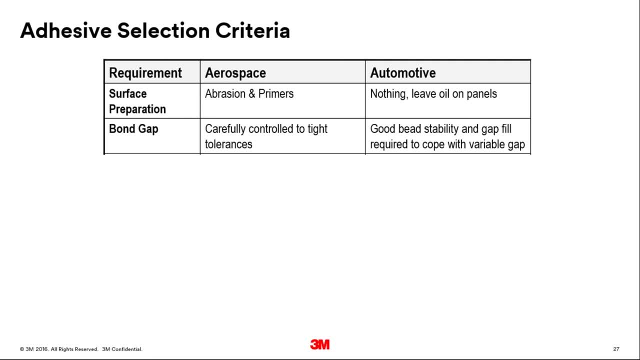 Required to cope with the variable bond gaps that the panel matches We'll provide. In terms of cure, we need to be very precise about cure cycles in ensuring that we get that hit, that level of performance promise for the adhesive in aerospace applications. 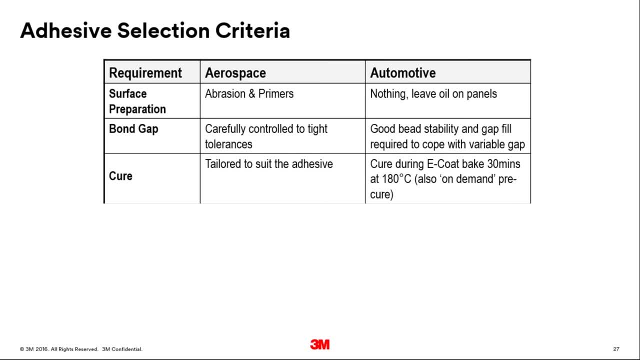 whereas automotive ask us to use their current cure cycle provided for the Ecote bake. The application environment for aerospace will quite often go into clean room standards, whereas automotive will want us to use their current production facility And we have much more time to apply our adhesive again. 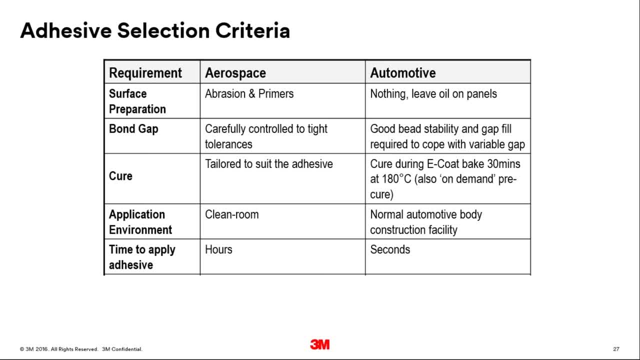 achieving that controlled bondline and ultimate performance, Whereas automotive will only give us seconds to apply the adhesive. And in terms of an inspection schedule, thankfully we have a regular safety inspection schedule in aerospace, Whereas in automotive it's left in the hands of 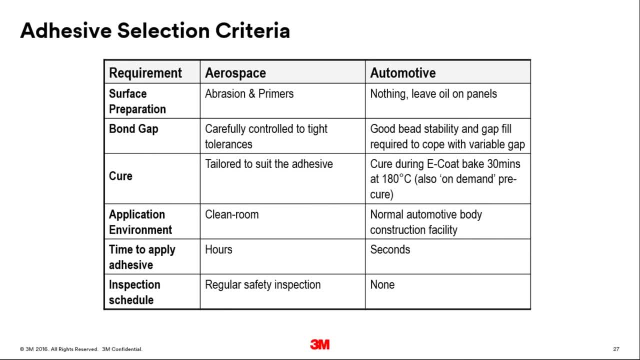 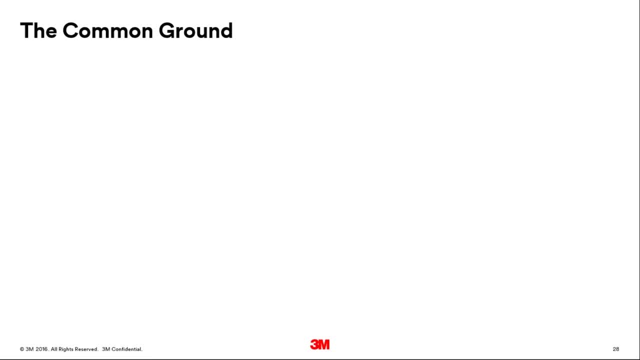 the final customer. But it's not all about differences. There's an awful lot of common ground. Both industries want to produce lighter structures at a lower cost, and faster cycle times are needed to hit the production volumes, Also looking for lower toxicity and safer. 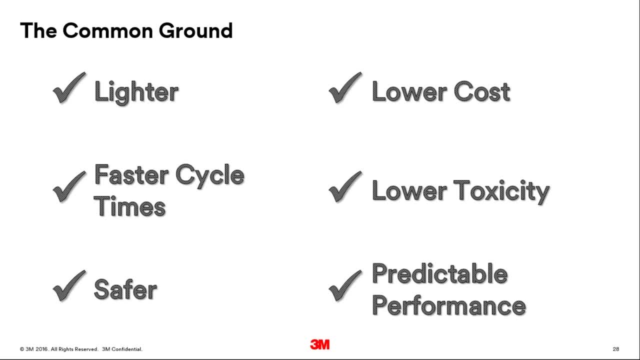 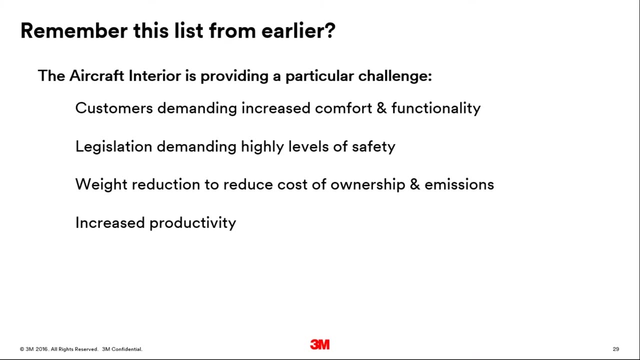 structures with more predictable performance as CAE becomes the mainstream- And hopefully you remember this list from earlier- that the aircraft interior is providing a particular challenge. There's a lot of common ground here with automotive. First of all, customers demanding increased level of comfort and functionality. Well, we're demanding that. 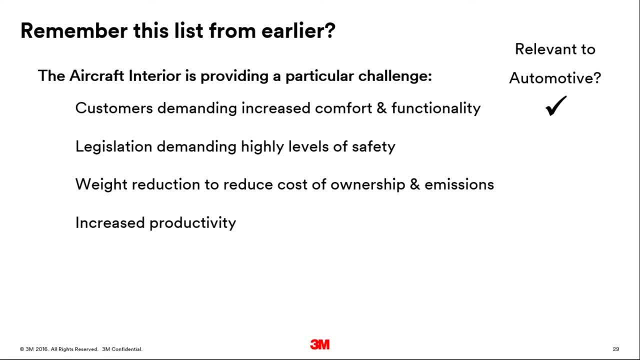 not only from aircraft, but also from our cars. Legislation is demanding higher levels of safety And there's also a weight reduction agenda in both industries to reduce the cost of the aircraft And there's also a weight reduction agenda in both industries to reduce. 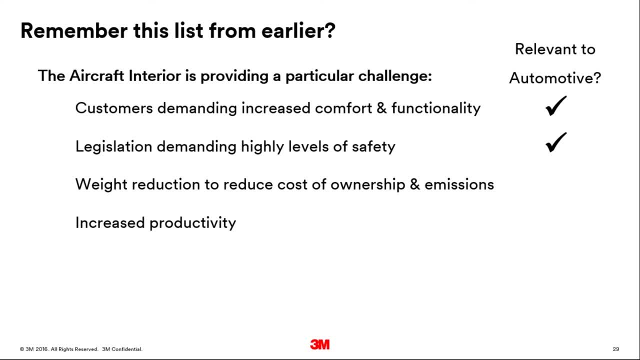 the cost of the aircraft And there's also a weight reduction agenda in both industries to reduce the cost of ownership and also reduce emissions. An increased productivity is needed in order to keep the cost manageable and keep the product going out the door at the rate that's demanded. 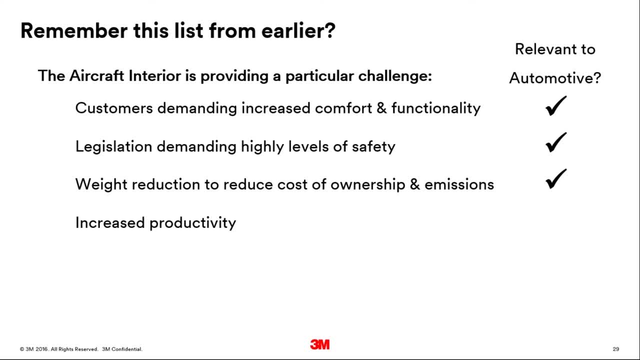 by the end customer. Now it's interesting for me, coming from an automotive background into aerospace, in that I'd not heard of FST in automotive. But having learned about that, it's certainly not going to be a surprise to me if FST becomes a requirement for automotive. 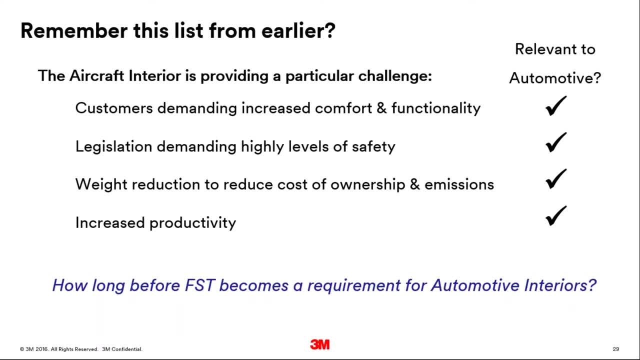 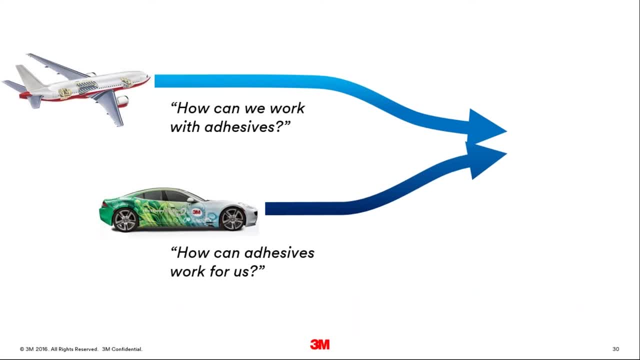 interiors. So it's clear that adhesives have a key role to play both in today's structures and in the planes and cars of the future. Major strides have been made by both industries, but in different areas: Aerospace- in terms of driving, the performance of adhesive systems- and automotive. 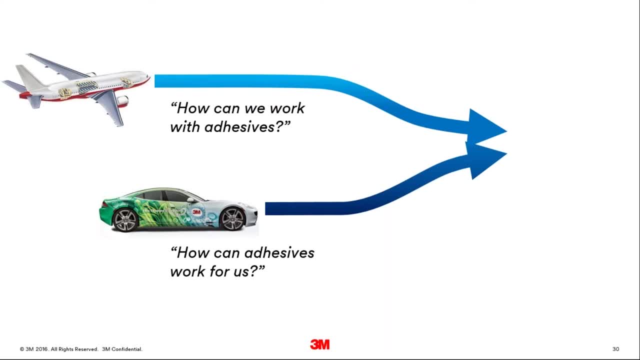 in terms of production methods and making the use of adhesives much more efficient. The flow of in information is clearly not one way. Both industries are keen to learn from each other, and indeed other industries are reaping the benefit from both the aerospace and automotive pioneers. 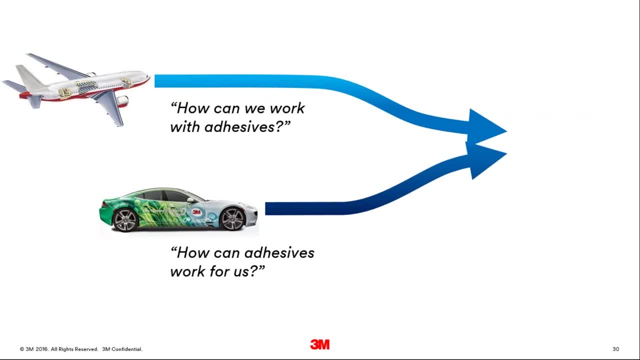 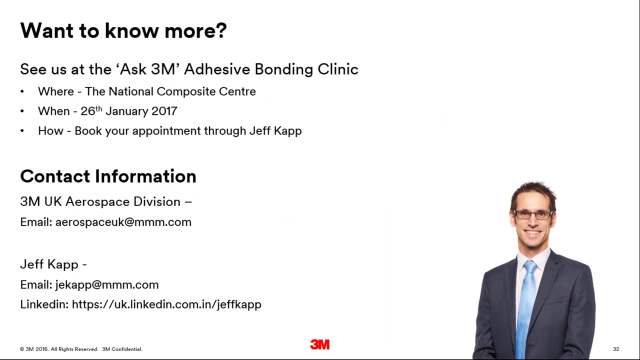 It's a great time to get stuck into adhesives, if you'll pardon the pun. We've achieved a lot, but the great prizes are still ahead of us. So today I've shared some of our journey over the last few years. I hope that you found it both in. 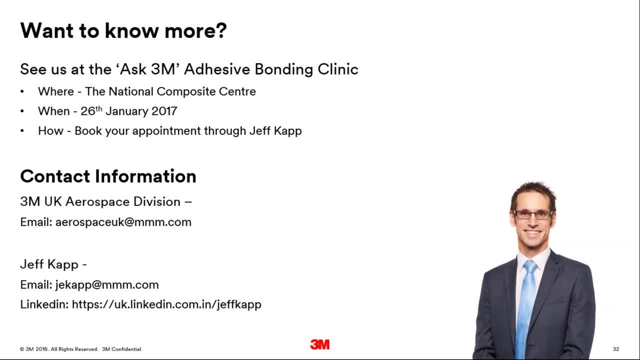 informative and inspiring, But if you'd want to know more, we're actually running an Ask3M adhesive bonding clinic. We're doing this at the National Composite Centre on the afternoon of the 26th of January And you'll be able to book 20 minutes appointments with me and also my colleagues. 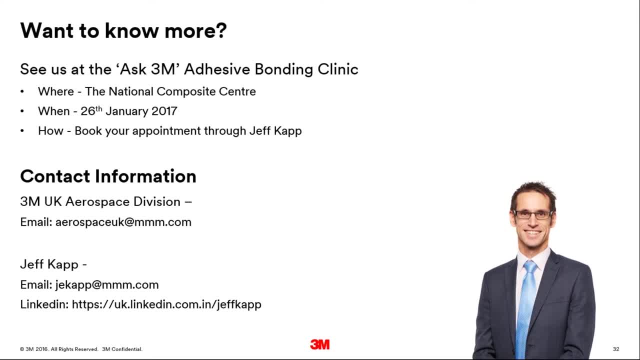 Bernard Sickle and Andrew Marks. If you'd like to contact me through any of the methods listed below, that would be great. Also, I think we've got time a few minutes today if you'd like to ask some questions online. If you'd like to contact me through any of the methods listed below, that would be great. But also, I think we've got time a few minutes today. if you'd like to ask some questions online. 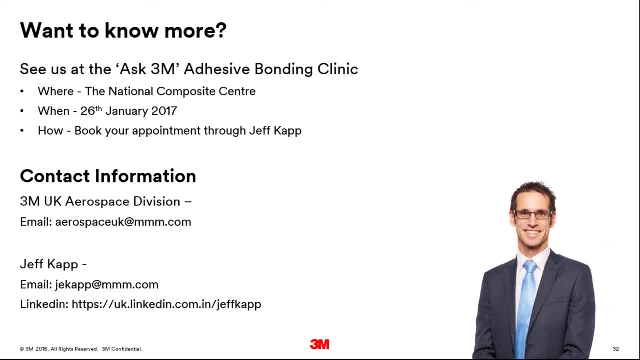 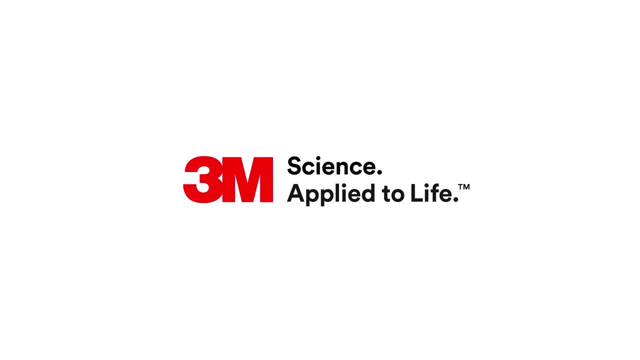 Okay, So we've had a few questions come in, One specifically about how adhesives can play a part in durability and NVH. very nice question. thank you very much for that. and there's actually been some studies done on this- that an adhesively bonded vehicle gives a noticeable improvement in terms of both the 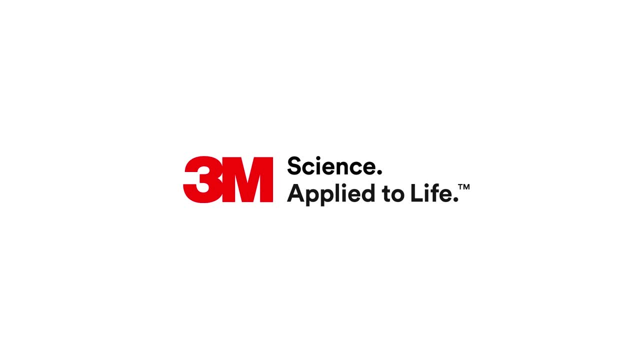 durability. so this is retained torsional stiffness and also noticeably quiet vehicle. quieter vehicle is achieved now. there's two reasons for this. the continuous bond, the continuous joining of, provided by diseases versus spot welding, actually changes the MVH response of the vehicle body. but also in retaining torsional stiffness you'll reduce the squeak and rattle that is developed through the 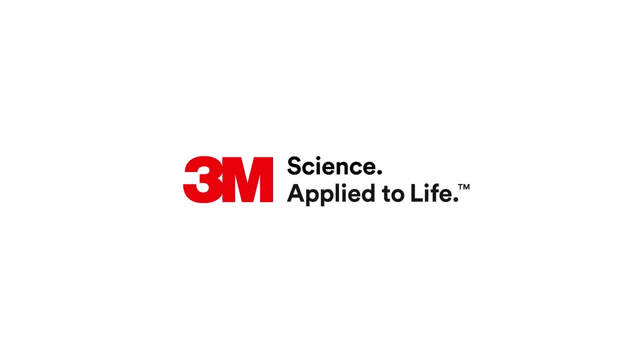 vehicle flexing. hopefully that answers your question. if you need to know a bit more, then please get in touch. okay, there's that. there's another question, come in and in. in terms of which is the most demanding- aerospace or automotive? well, I would actually say that they're both as demanding as as each other. 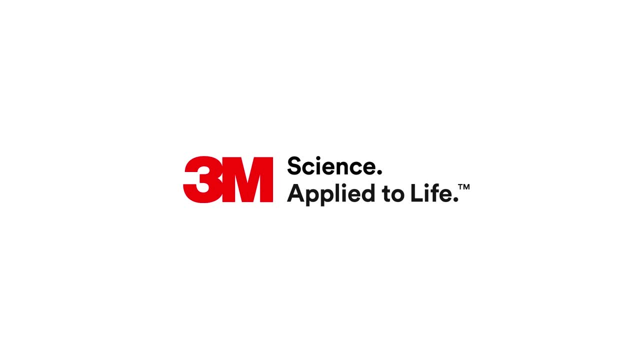 but in different ways, and the levels of performance that we need to need to achieve in in aerospace is extremely challenging, but at the same time, in automotive the kind of cycle times were given and the, the substrates that we need to bond to our just as challenging 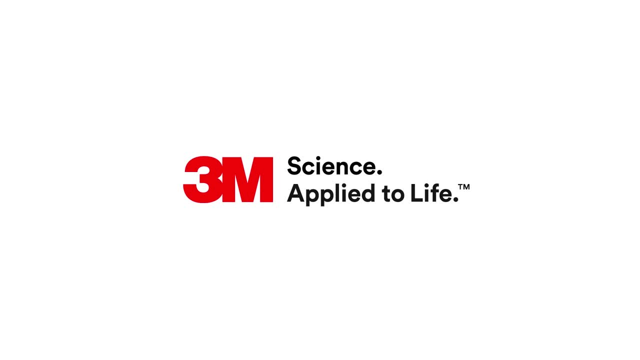 there's. there's a question come in regarding stable, stable beads and ability to respond to all the surfaces. are there any plans to make these aerospace qualified? As I highlighted, both industries are learning from each other And certainly we are seeing interest in this kind of robustness approach of automotive coming over into aerospace. So I can't. 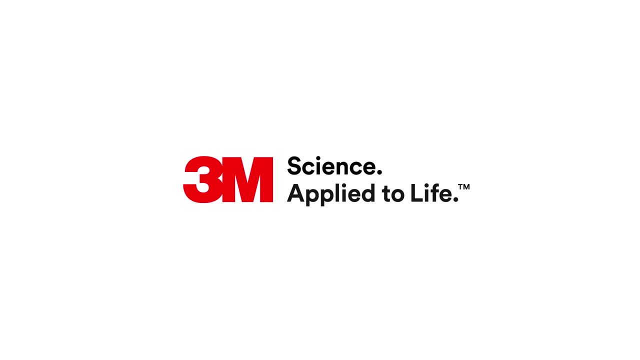 answer that question specifically, But generally, yeah, we're seeing lots of overlap between the two industries. Okay, and somebody's asked if we can get a copy of the presentation. I think that is yes, that's going to be shared. 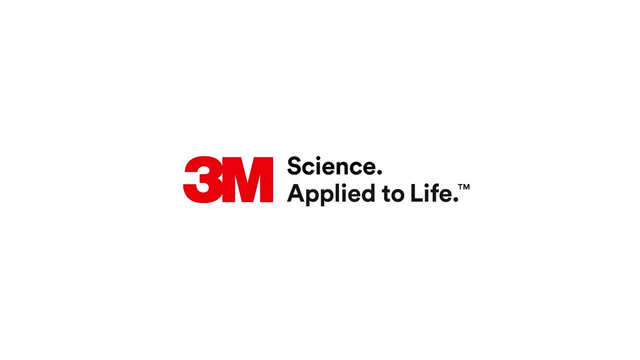 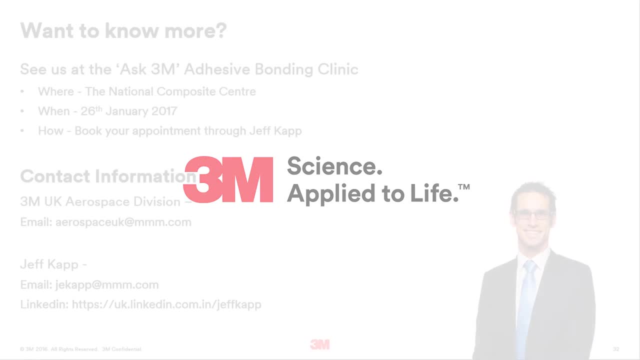 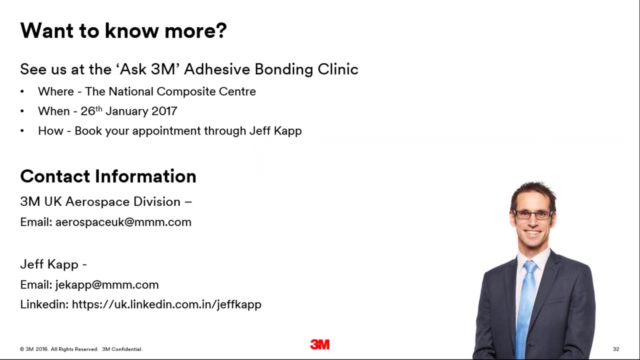 So my email address- I'll just put the slide back up- is jecap j e k a p p at nn. mcom. of course, find me on LinkedIn. So thank you very much for today. I hope you found this interesting and informative. 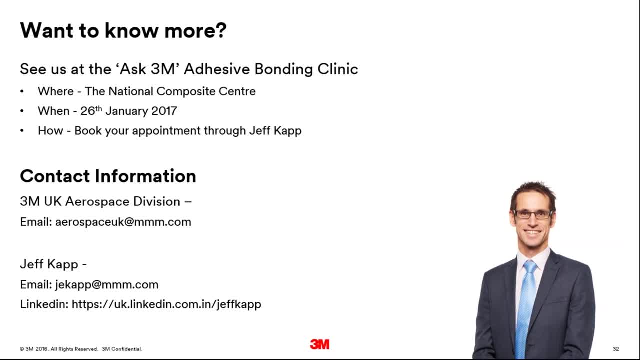 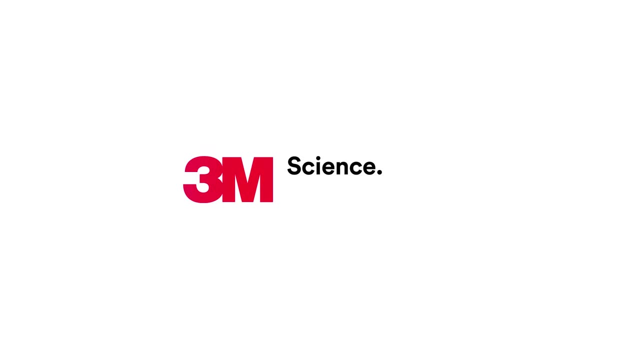 and, in some ways, entertaining. Enjoy your wine down to Christmas, if indeed you're at that point. if not, I hope that you get everything done before you go off for Christmas. Take care, you.